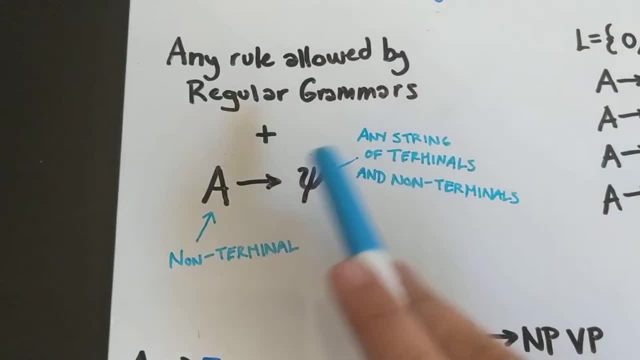 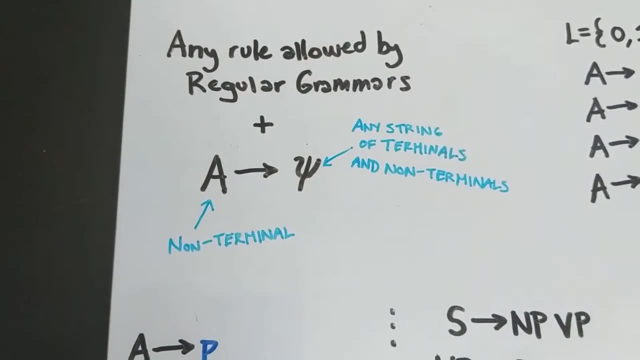 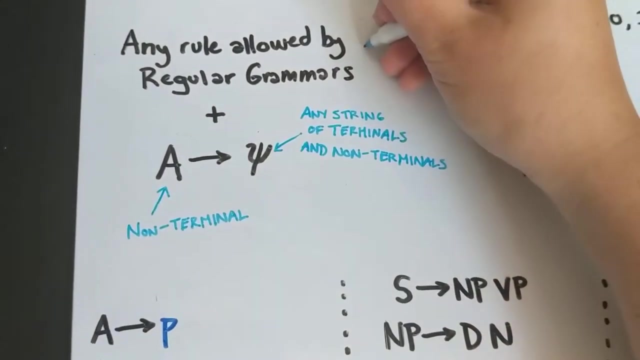 a couple videos from now. All right. so what is this format of a rule? This says that any non-terminal node is made up of a string of terminals and non-terminals. So remember that when we were talking about regular grammars, the right side of these rules could only be a single non-terminal followed by a terminal. 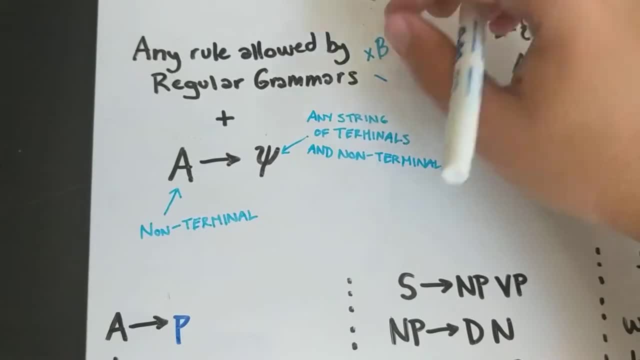 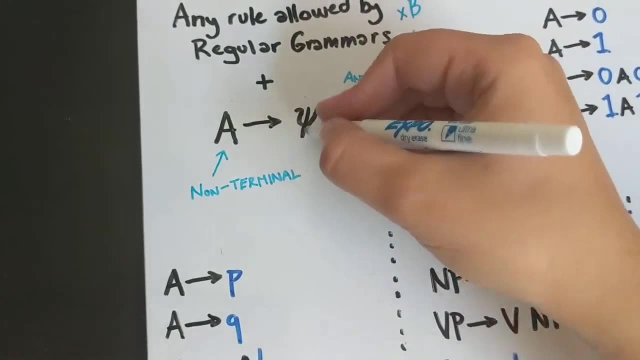 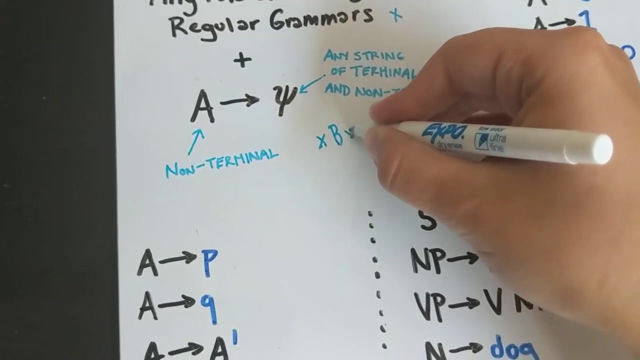 or it could just be: or a single terminal followed by a non-terminal, or it could just be a single terminal, right? So this is different from any string of terminals and non-terminals, right? So this could be, you know, a non-terminal followed by, or terminal followed by a non-terminal followed by. 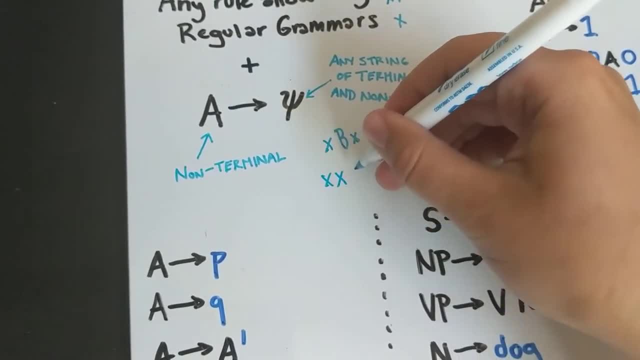 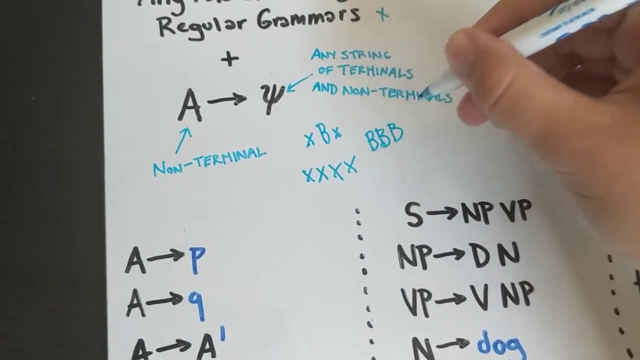 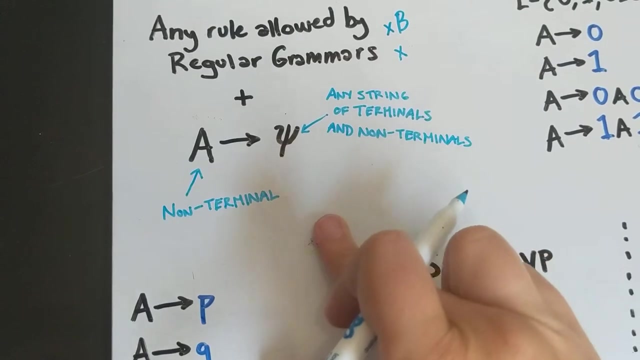 a terminal. It could be four terminals in a row. It could be three non-terminals in a row. right There's a lot more flexibility on what can be on the right side of rules of this type. The place where there still is not flexibility is on the 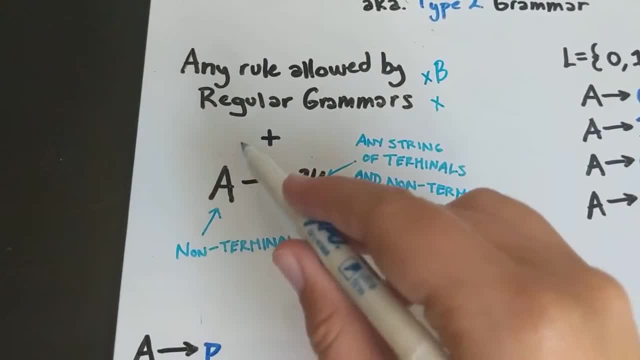 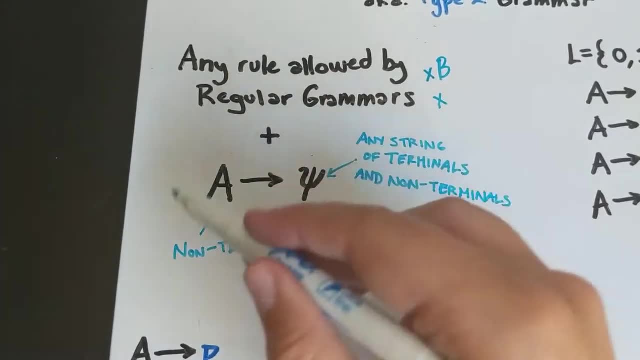 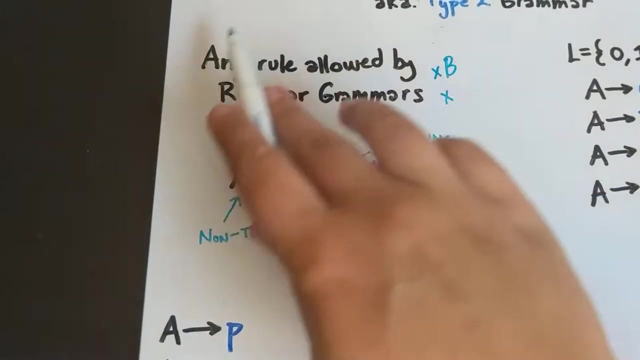 left side. So notice that the left side of these rules has to be only a single, non-terminal right. So that's where we still don't have the full extent of what our definition of grammar rules allows us to put on the left side right. So this is: this is a context-free grammar. 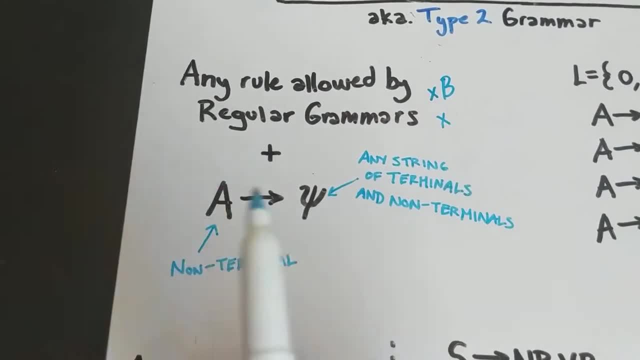 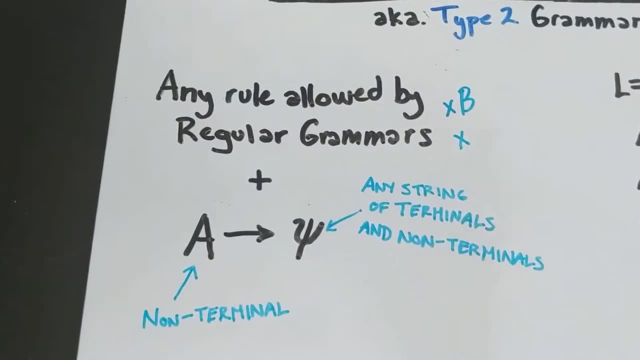 Any rule allowed by regular grammars, and then any rule that is a terminal made. that means that a terminal is or non-terminal, is made up of any string of terminals and non-terminals. So let's look one more time at the example that we were talking about in the video about 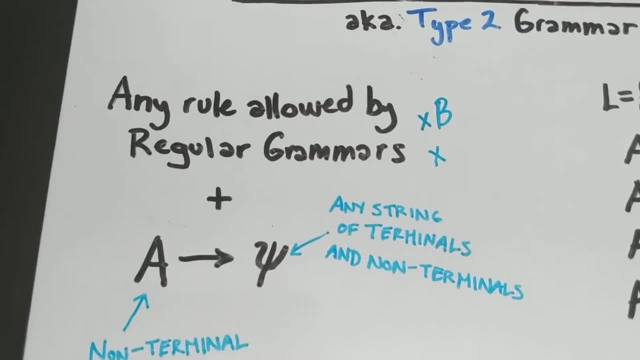 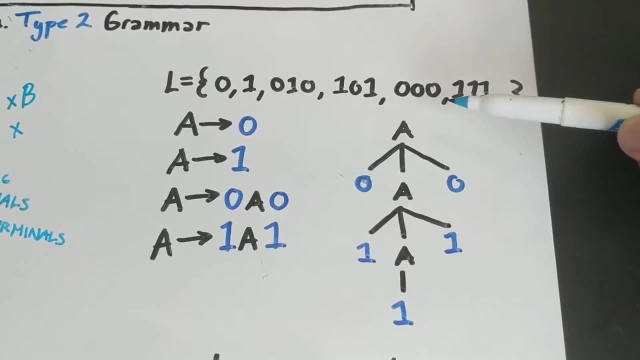 regular grammars, and we'll walk through this example of a context-free grammar. So this is a context-free grammar. So this is a context-free grammar. So this is a context-free grammar. This is the language that is made up of any string of ones and zeros, So that it's read: 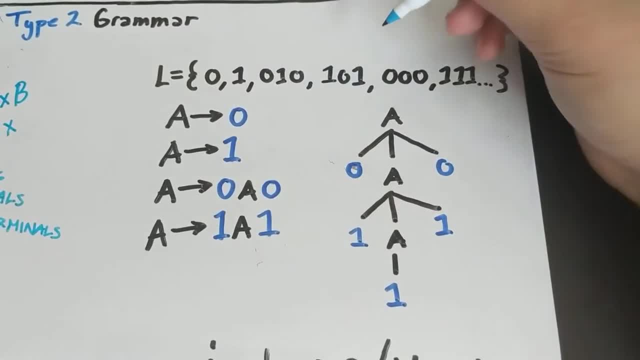 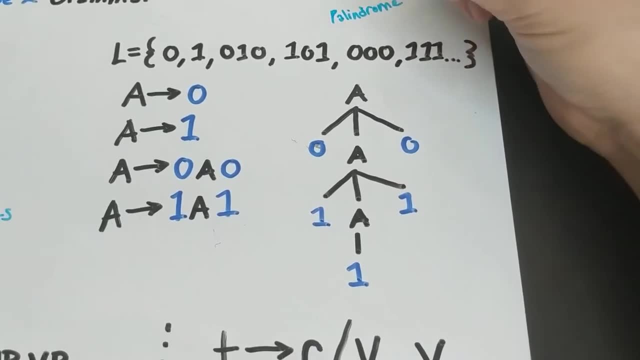 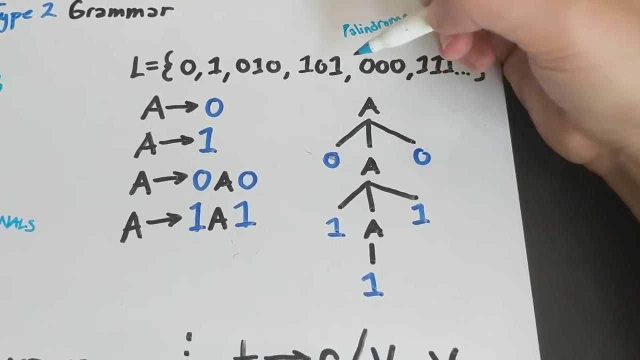 the same forward as backwards, right? So this is a palindrome language. That's what these are called: palindromes, right? So 0 0 0 is the same as 0 0 0,. 1 0 1 is the same as 1 0 1,. 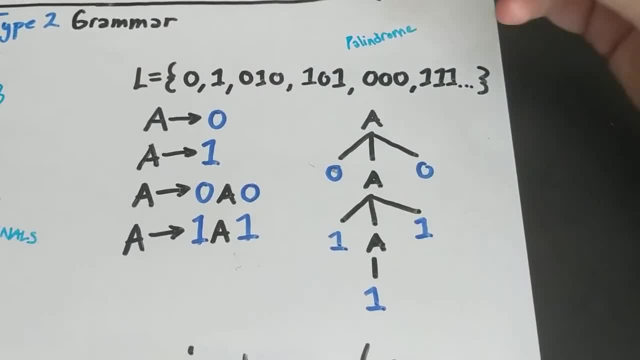 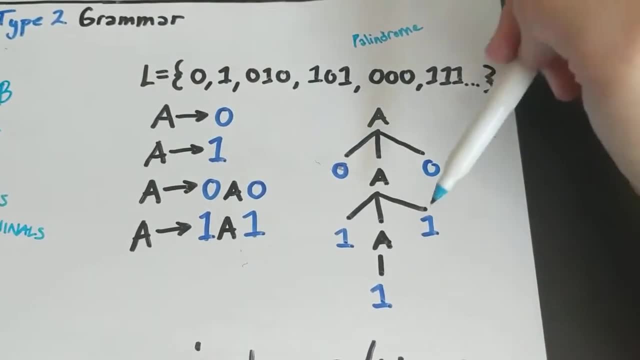 right, so on and so forth. And in the last video we explained why we cannot account for this using regular grammar rules, and in this video we're going to talk about how we do account for it using a context-free grammar right, so we can have a rule of. 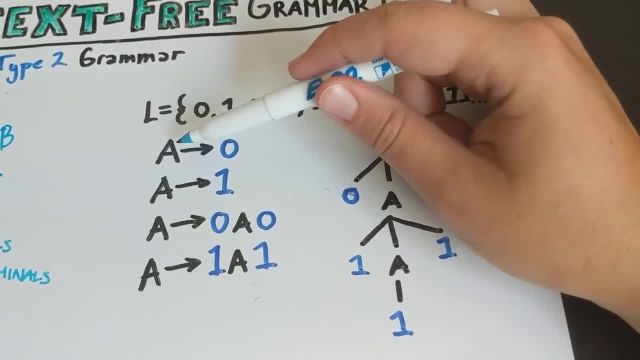 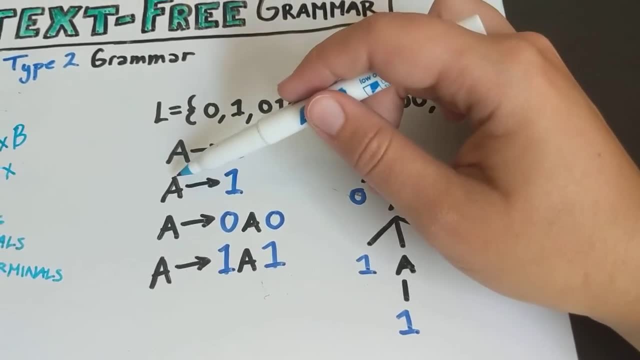 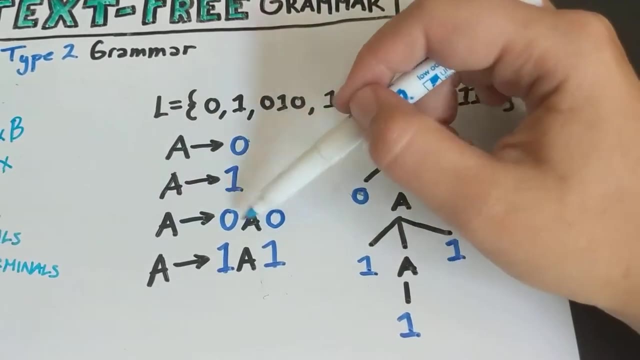 this type right. we have. a single non terminal is made up of a terminal which is a string of terminals and non terminals. this is any. a non terminal is made up of a string event of terminals and non terminals. this is right. so these all fit into our context-free grammar rules and they will also generate your. 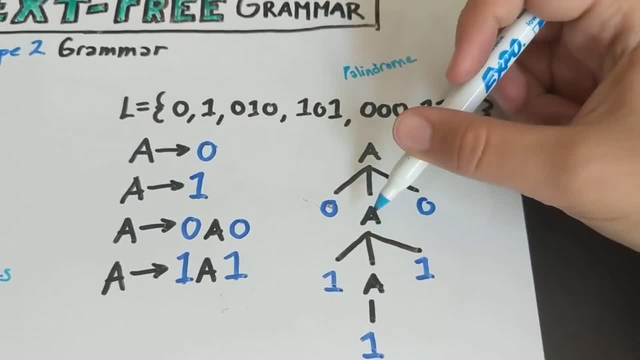 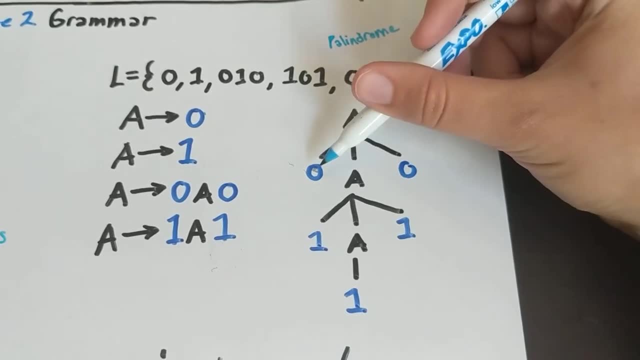 palindrome language right, so a is made up of 0 a 0, a is made up of 1 a 1 and a is made up of 1 right, so this generates a string: 0, 1, 1, 1, 0, which is the same as. 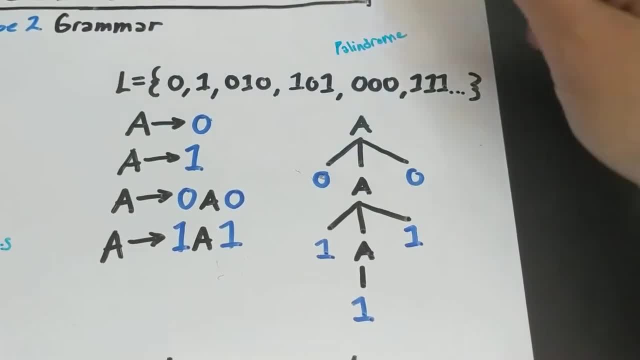 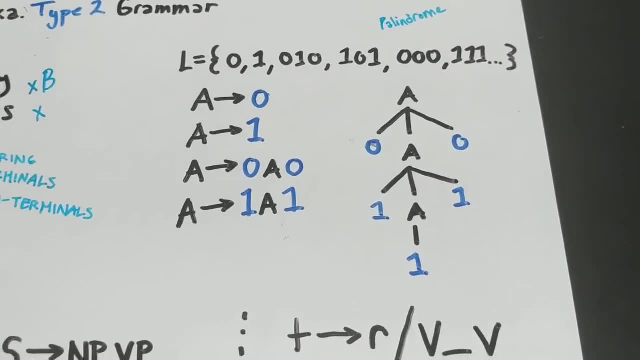 0, 1, 1, 1, 0. right, so that's how we use a context-free grammar. let's walk through a couple more context-free grammars that we have created so far or talked about- or you may have talked about in other classes. so we definitely have spent a lot of time. 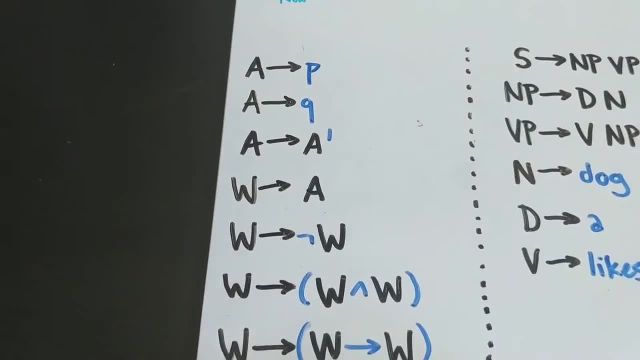 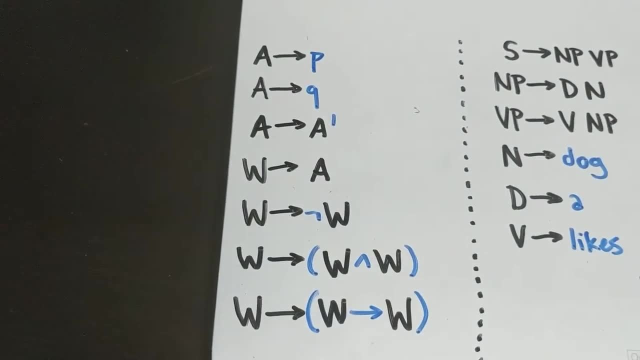 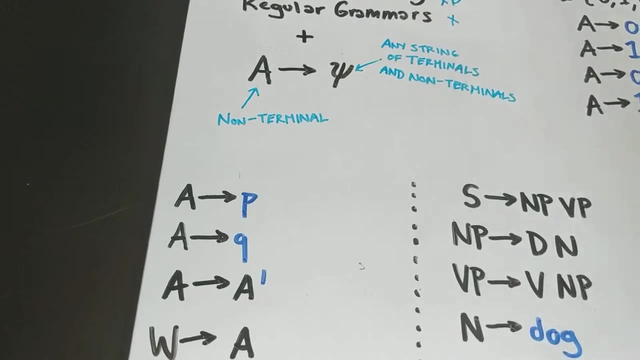 working with this one. this is just. this is not all the rules, but this is some of the rules of propositional logic, right? so some of these rules would be allowed by a regular grammar. so let us highlight which of the rules here are allowed by a regular grammar. this rule here: that's perfectly fine according to a regular 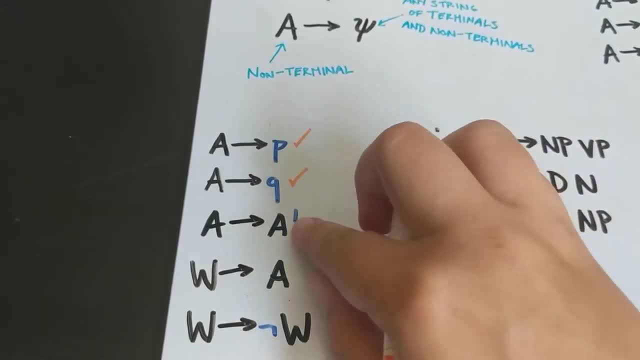 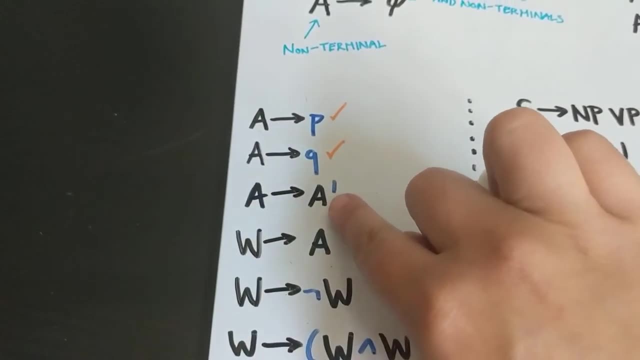 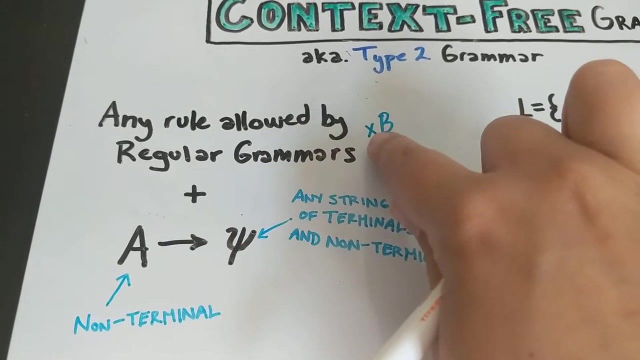 grammar, this is perfectly fine according to a regular grammar. then we look at this one, right? so this is a non-terminal, is made up of a non-terminal followed by a terminal. this is not allowed by a regular grammar, right? a regular grammar says you have to have a non-terminal or a terminal followed by a non-terminal. 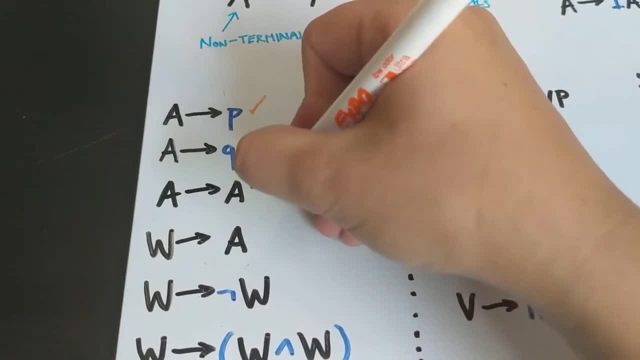 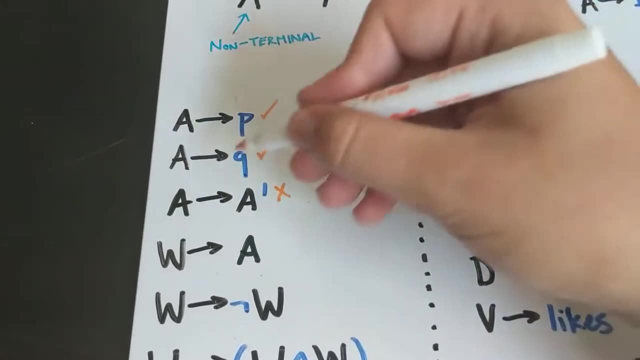 that's the wrong order here, so this is not allowed by a regular grammar. this requires that we're using a context-free grammar to have this rule at all right. so that seems fairly simple, but you're not allowed to have this rule if you're. if you're. 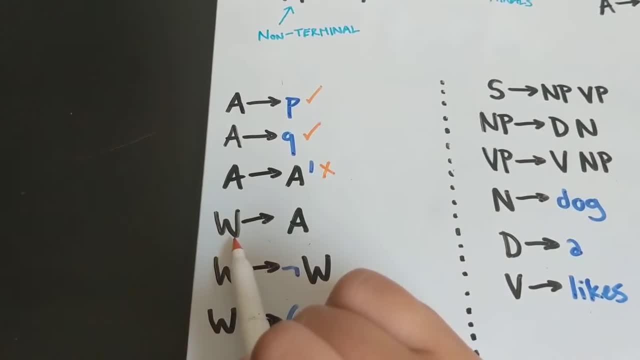 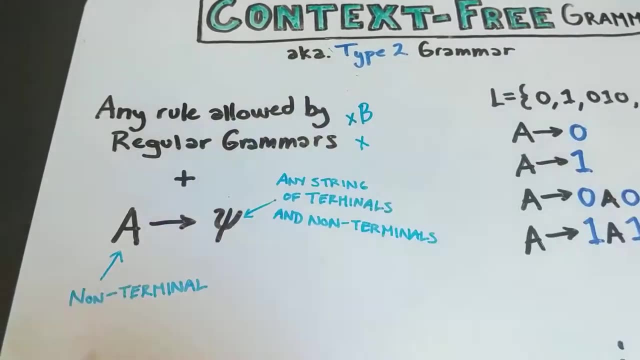 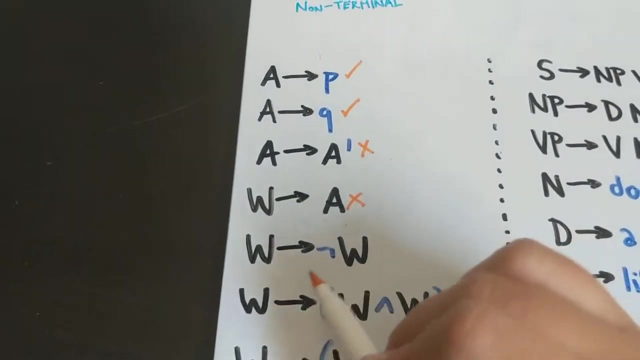 making a regular grammar. How about this rule? A non-terminal is made up of just a non-terminal. Is that in our list for regular grammars? No, it's not. So this is not allowed by regular grammars, right? So we already have to be using a context-free. How about this one? 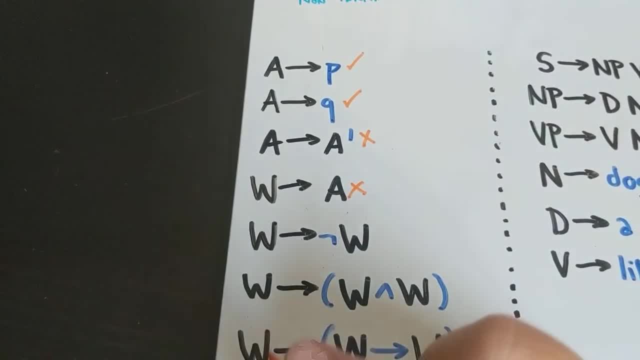 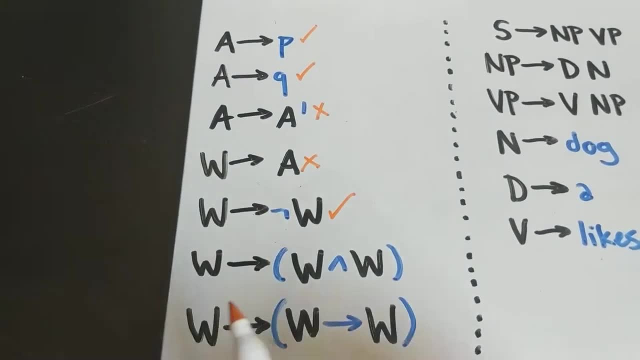 A non-terminal is made up of a terminal followed by a non-terminal. That's totally fine according to regular grammars, right? That's just this. So this is a rule that you could do. How about this rule? Totally not okay according to a regular grammar. We're not even going to go back, and 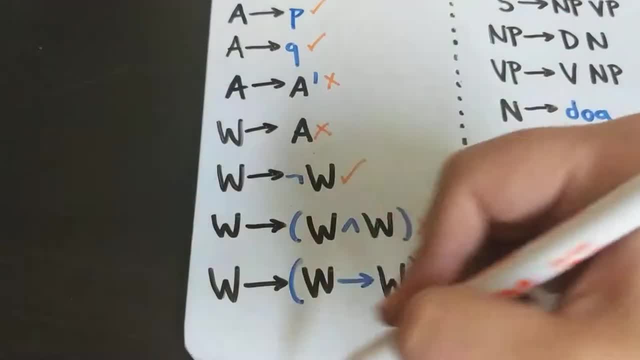 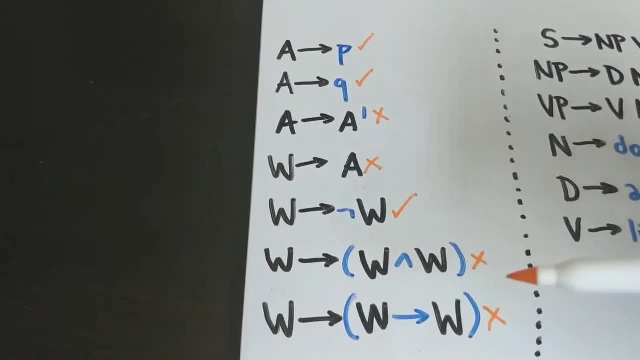 look at those definitions, And this one too, right? So these are both. these are all requiring that we are using a context-free grammar. So the grammar that we have come up with for propositional logic is a context-free grammar. All right, here's another one that you might be. 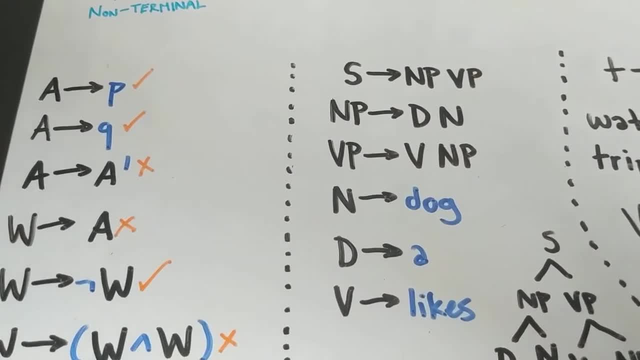 familiar with. if you've taken a linguistics class before. I know that not all of you have taken one. I know that not all of you have taken one. I know that not all of you have taken one. You've taken linguistics classes before, but this is actually a context-free grammar. These 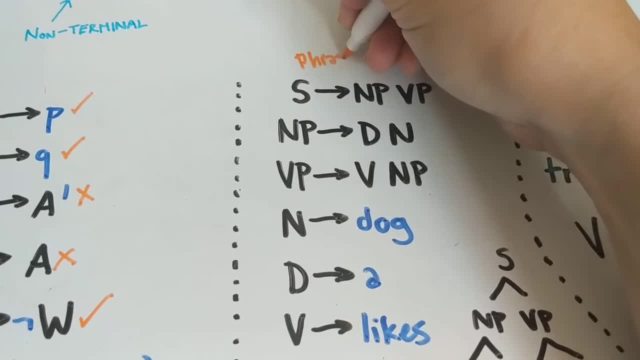 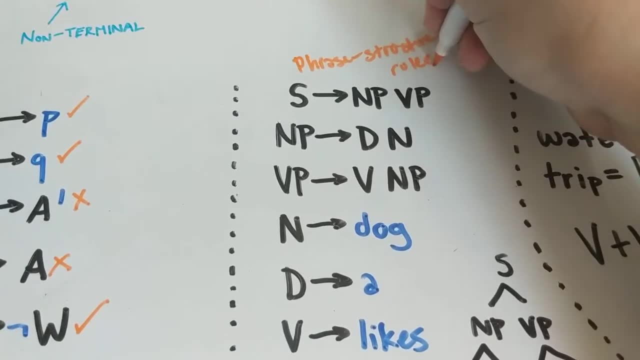 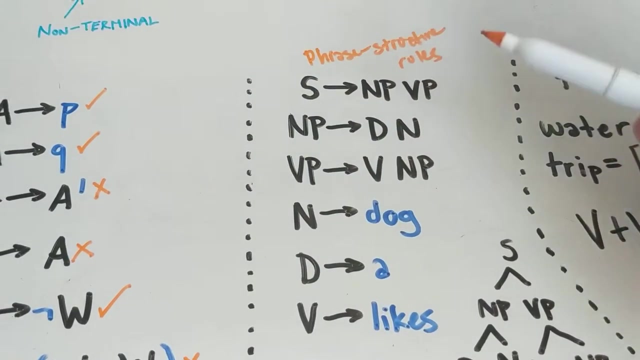 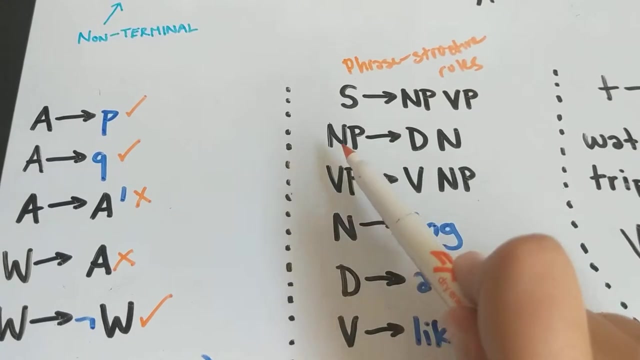 are called phrase structure rules, And they're what we use to evaluate whether the syntax of a sentence is grammatical or not, right? So this means that a sentence is made up of a noun phrase followed by a verb phrase. These are non-terminals, all non-terminals. 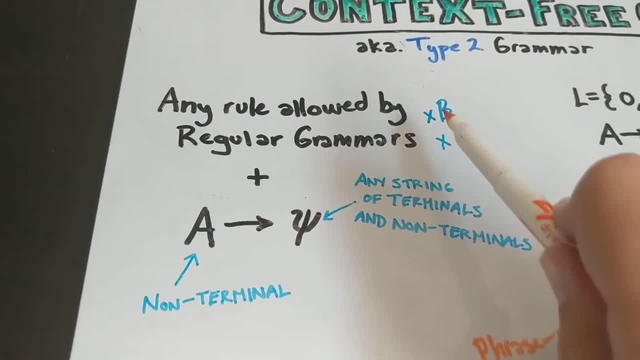 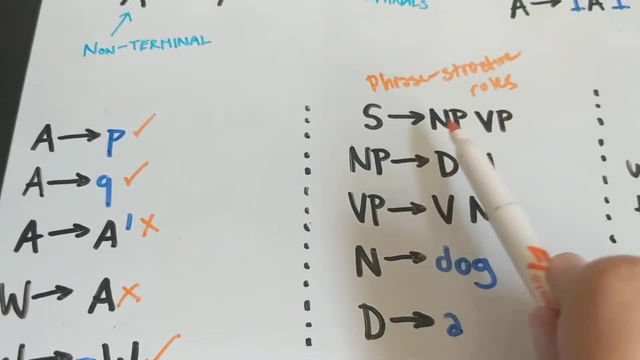 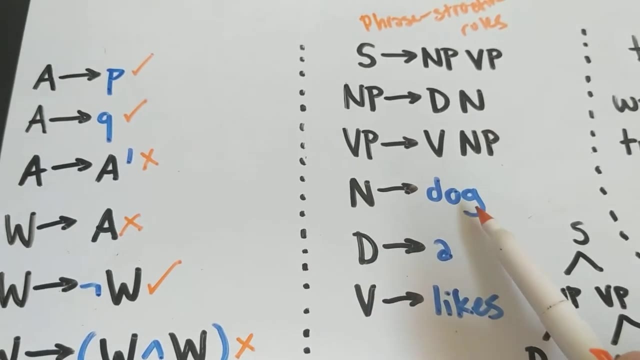 right. So this could not be in a regular language because we don't have a non-terminal. in this rule, A noun phrase is made up of a determiner and a noun. Still, we're working with non-terminals. A verb phrase is made up of a verb and a noun phrase. A noun is made up of dog can be a dog. 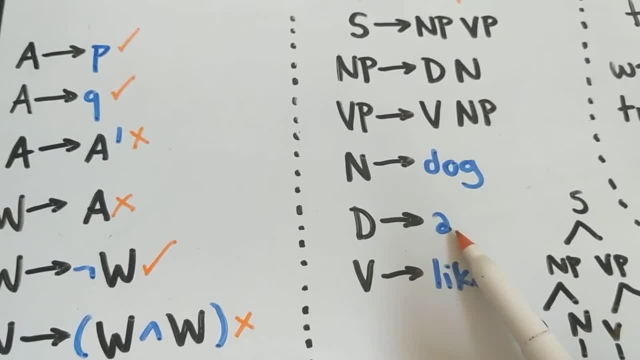 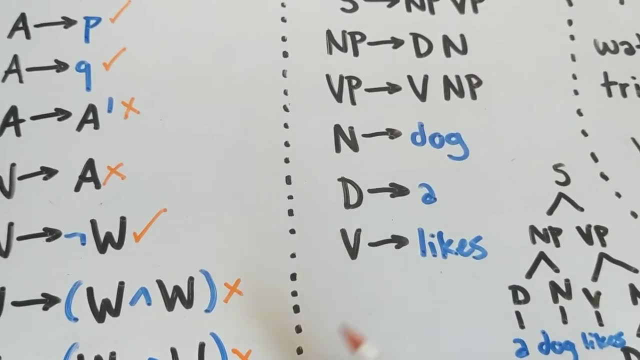 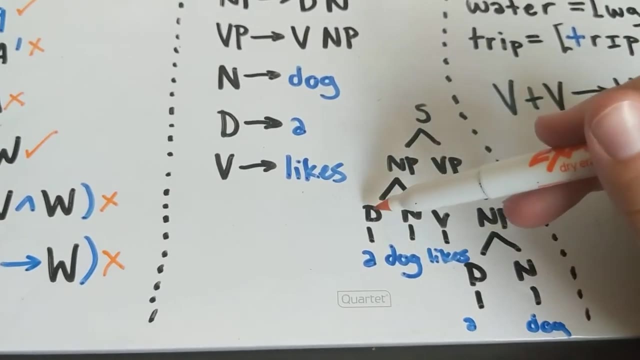 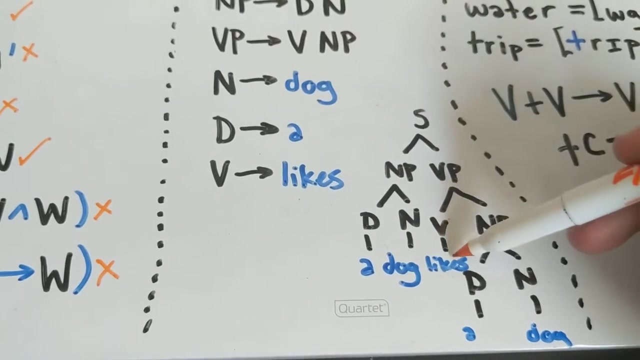 which is a terminal. A determiner can be a, which is a terminal in this case, And a verb can be likes Terminal. this allows us to generate this whole structure. here A sentence is a noun phrase and a verb phrase. A noun phrase is a determiner and a noun And a determiner is a. A noun is dog A verb. 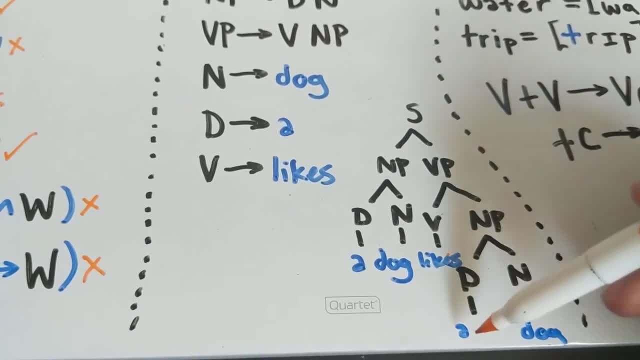 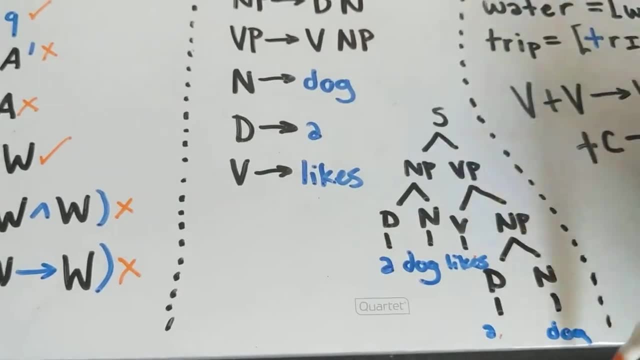 is likes A noun phrase is a determiner and a noun. A determiner is a And a noun is dog. We can generate a sentence: a dog likes a dog. This is a very boring sentence, but we can use just these. 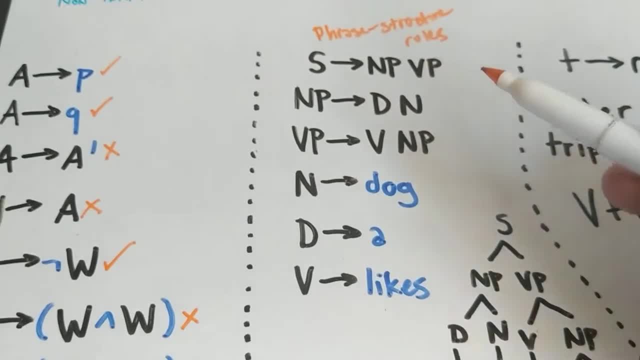 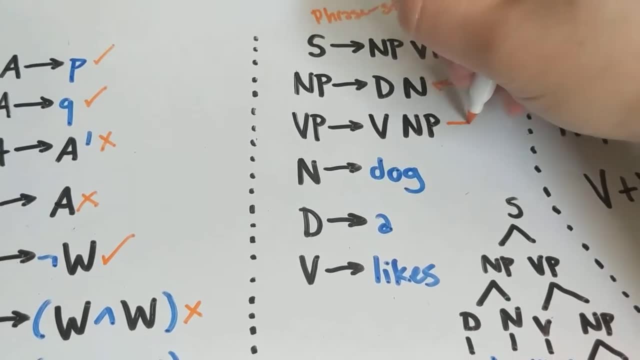 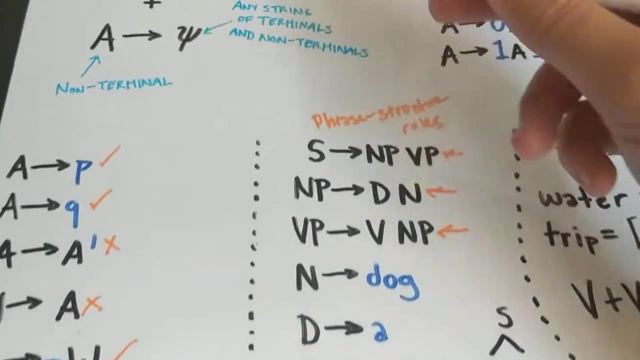 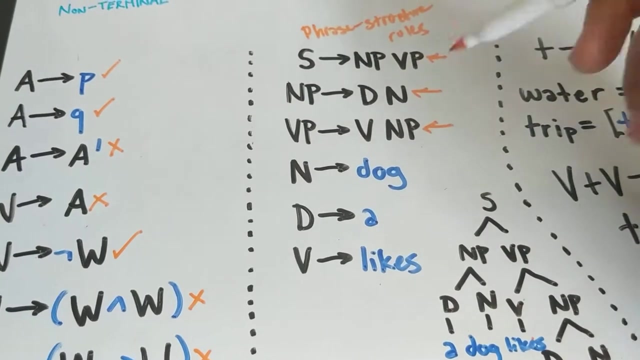 rules to generate this, But it is also a context-free grammar, as we note by these things. Now there's people, because context-free rules are more complicated than regular grammar rules. if you've taken a syntax class, you know that as syntax moves on, people tried to. 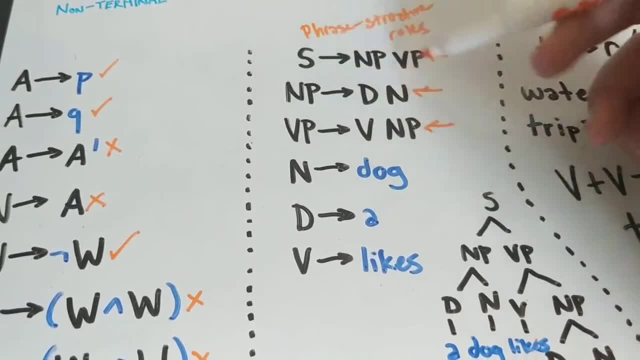 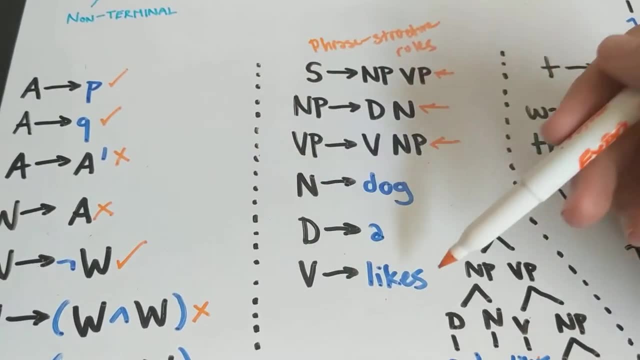 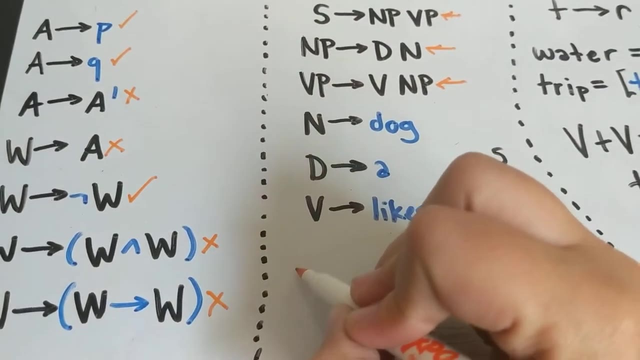 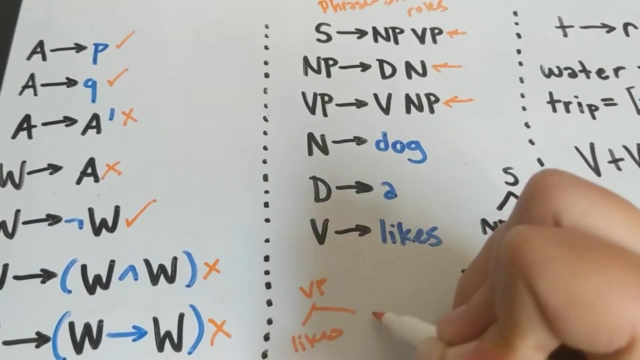 have tried to make as many of these style rules into these style rules as possible to make the grammar Simpler. So that is what we're doing when we when we switch up those rules. So if you take in a syntax class or linguistics class before, that's what's going on when people prefer to have a rule that's like verb phrase goes to likes noun phrase rather than you know something more complicated. 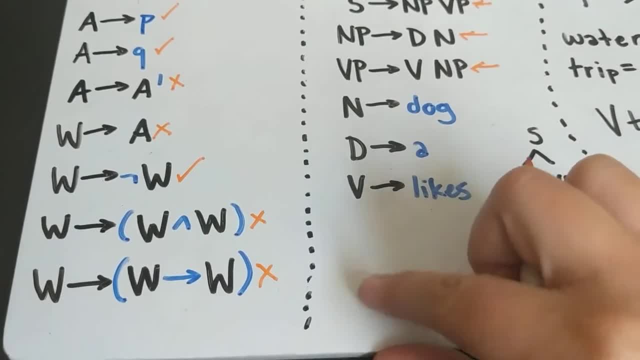 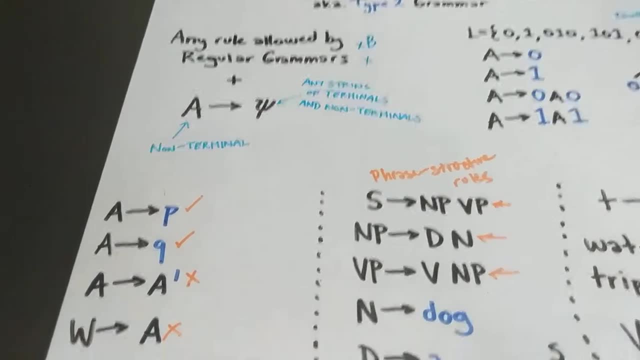 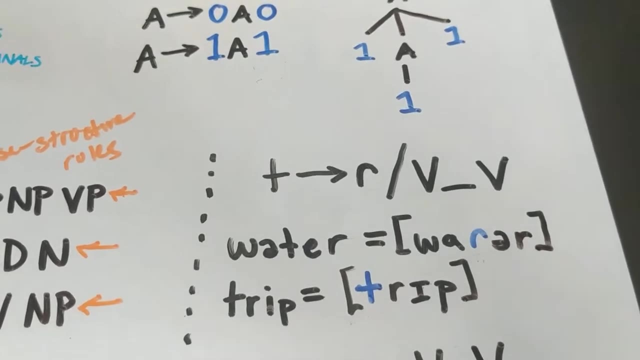 All right, Now let's talk about a thing in linguistics that we can't really model so easily with just context-free grammar rules, And this is something from phonology which you might not be familiar with. You might be familiar with if you have taken a lot of linguistics classes. 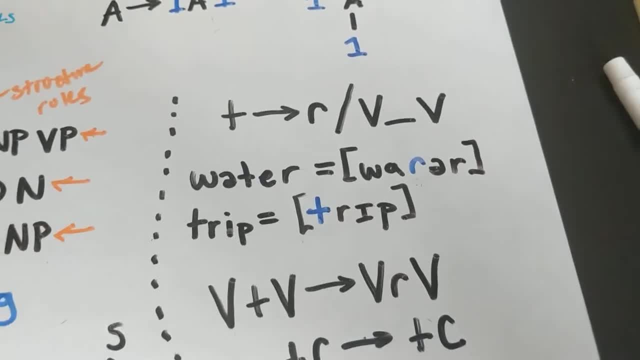 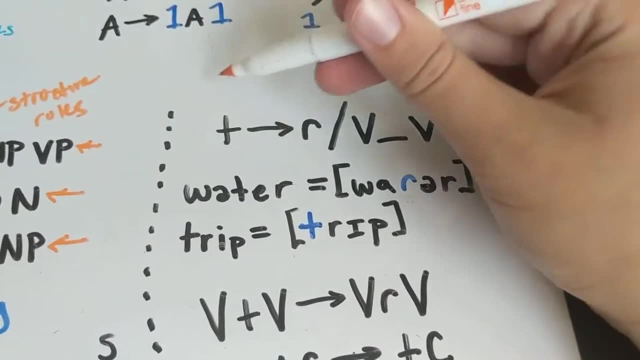 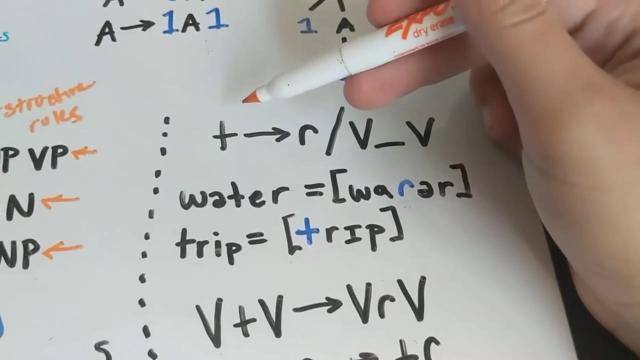 but we're just going to explain this example as though you don't know anything about this. So this is what we call a phonology, a rule of phonology, of the phonology of standard American English, right? So what does this say? 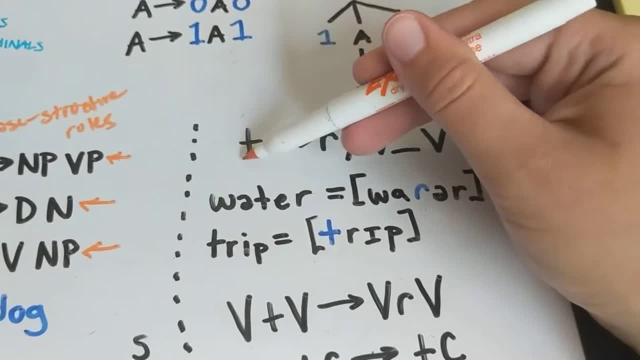 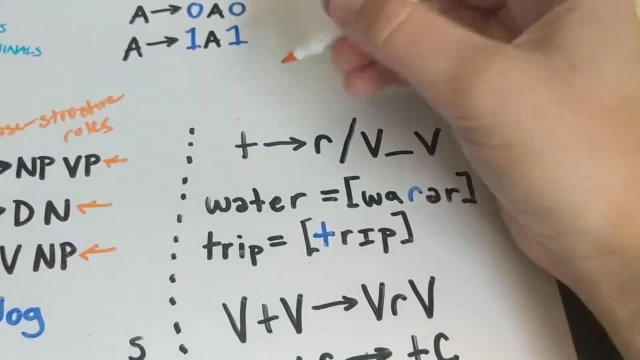 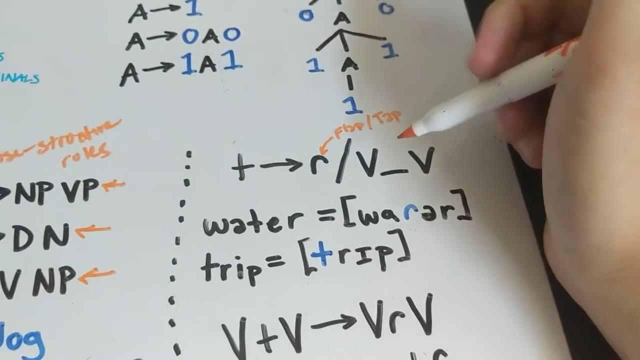 This says that any sound that we think of as being a T, which we, which is pronounced Tuh right, Any sound that we think of as being a T is pronounced as: this symbol, which is called a flap or a tap, is pronounced as this if it occurs between two vowels: 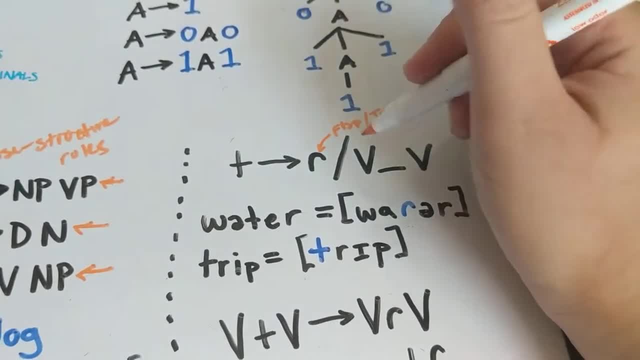 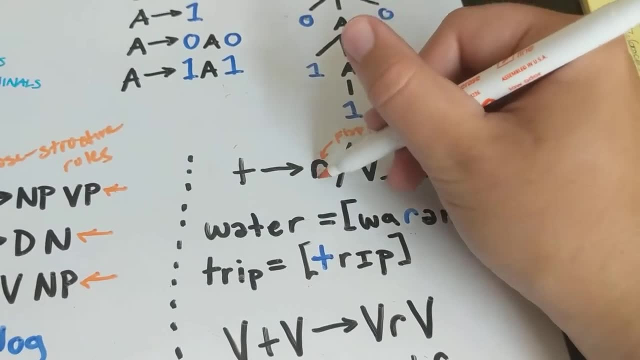 Actually it's between two voice sounds, but for this we're just talking about them as vowels. So this is. this is pronounced as Ruh. It sort of sounds like a D, but it but it's faster. This is the sound that R is in a lot of non-English languages, right. 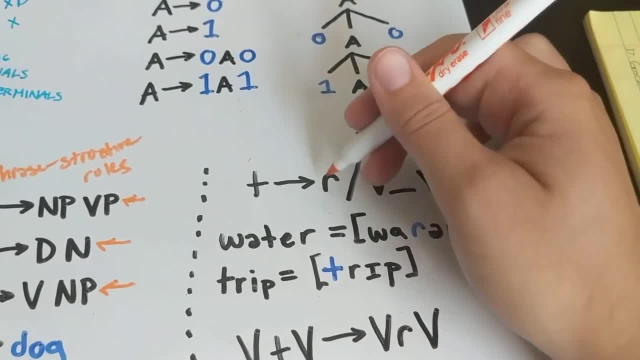 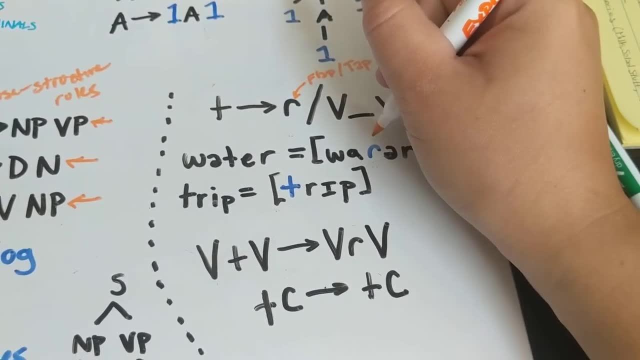 So this, this symbol, is a little bit like an R, It's a little bit like a D, but this is why, when we say the word water in standard American English, it's water, duh, duh. It sort of sounds like a D in there instead of water right. 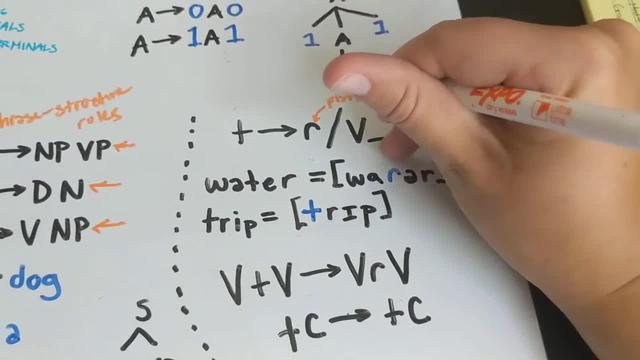 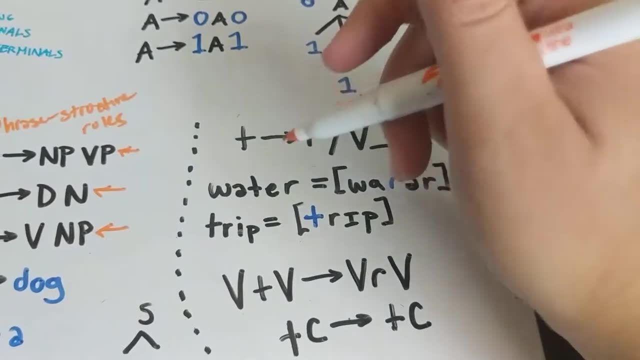 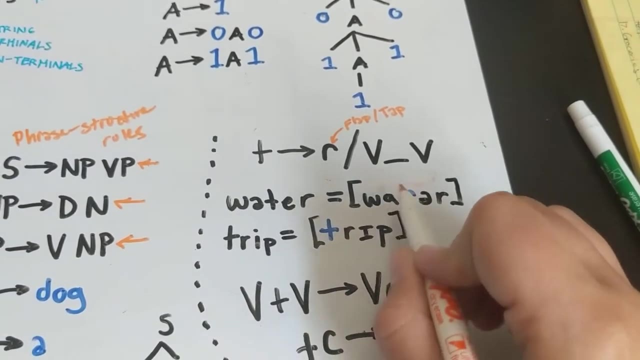 So in British English it would be a T, but in standard American English this gets flapped- is how you can say it- and it becomes water, water, right. But this doesn't happen to every T, right. It just happens to some T's when the T occurs between vowels or voice sounds right. 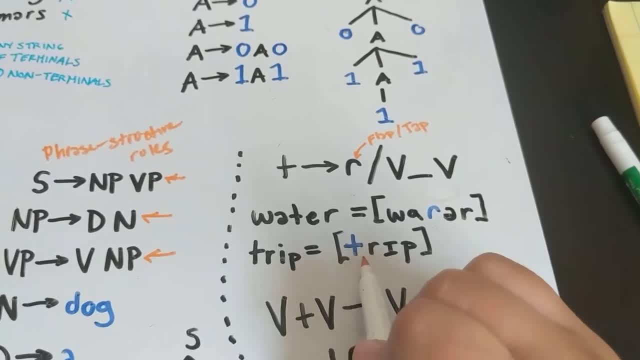 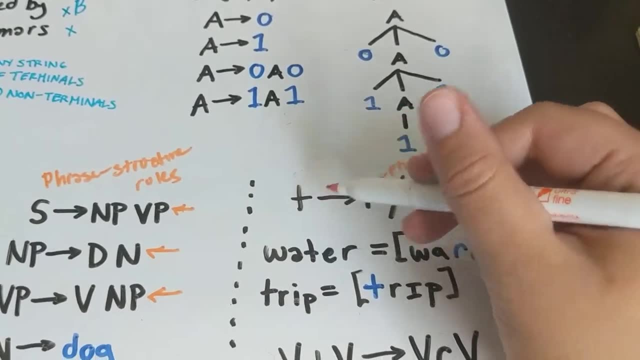 So in the word trip, for example, we still have a Tuh sound right, It still sounds like a T, right? So how do we represent a rule like this that says that that a T is pronounced as a Ruh? 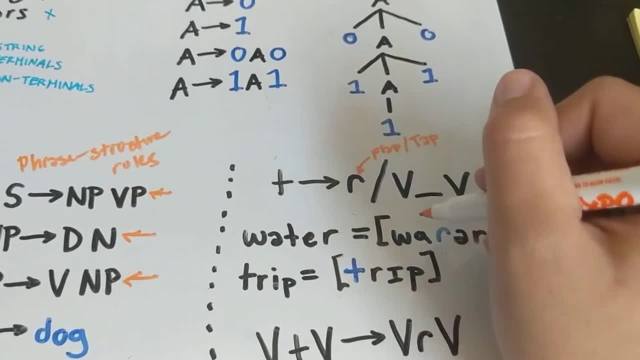 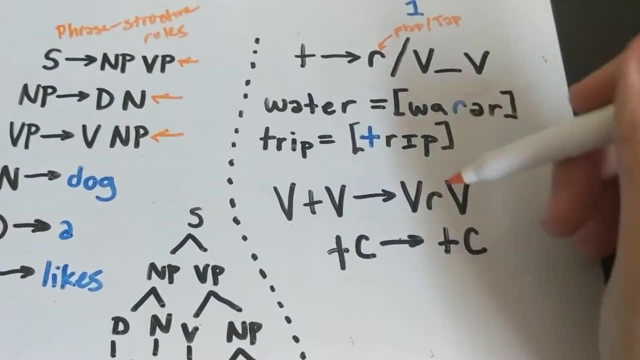 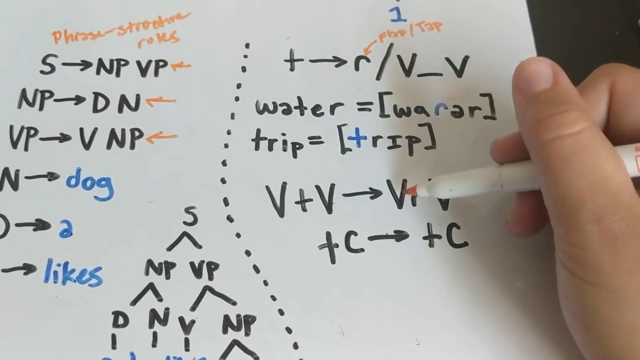 only in between vowels, but not elsewhere. right? This is something that's really hard to do with a context-free grammar. The best way to do it would be to write a rule like this that says: if you've got a vowel a T and a vowel that breaks down into a vowel, a Duh in a vowel. 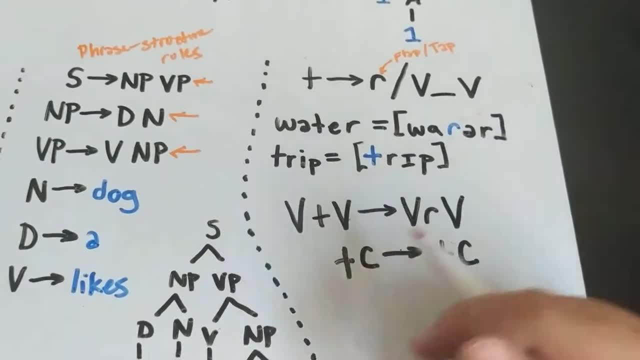 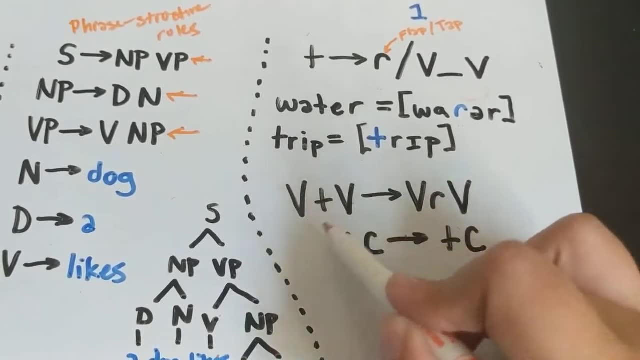 And then you could have other rules about T's in other contexts or just not break down your T right. So this requires that we have anything we want on the left side Right, Which we're not allowed to do with a regular grammar right. 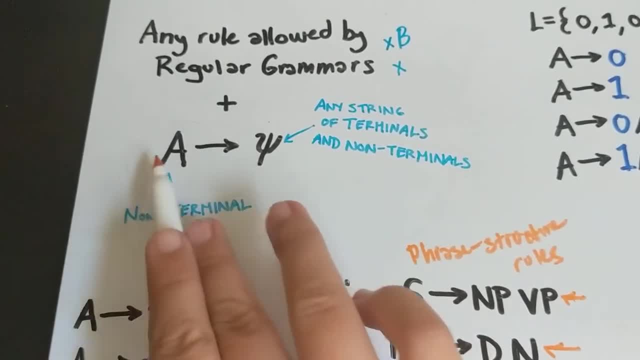 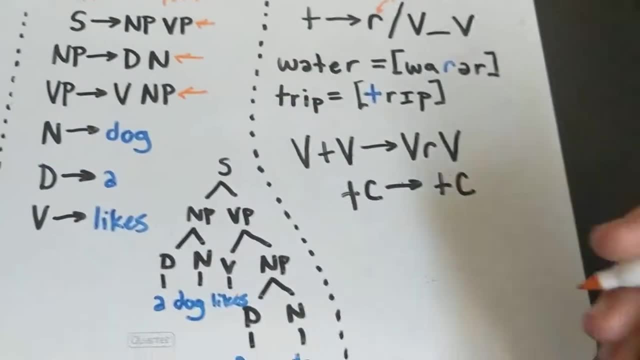 You're not allowed to put with a context-free grammar. you're not allowed to put anything you want on the left side. You can put anything you want on the right side, but not on the left side. Remember, our only rule for making grammar rules was that you have to have a non-terminal on the left side, right. 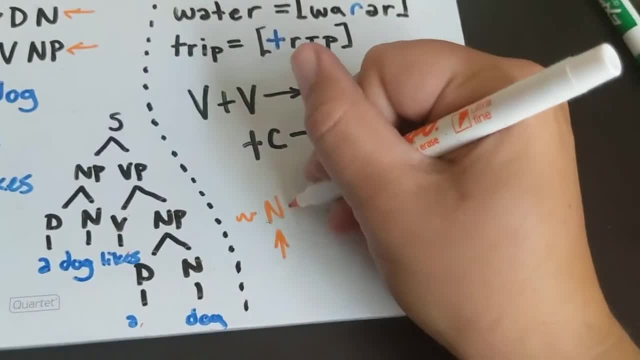 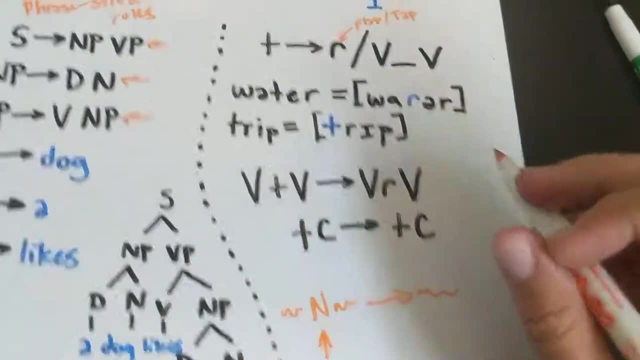 So you have to have a non-terminal, but then you can have anything you want here, anything you want here and anything you want here, right? The only rule is that there has to be a non-terminal on the left side, right. 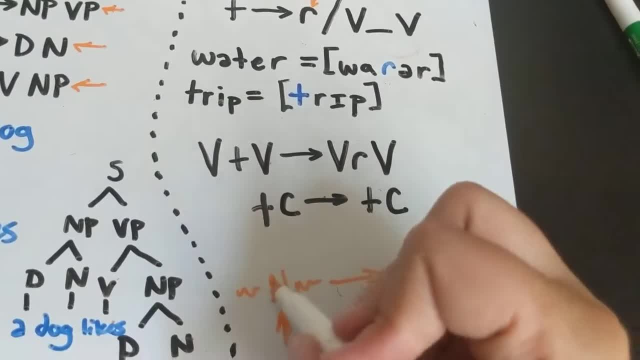 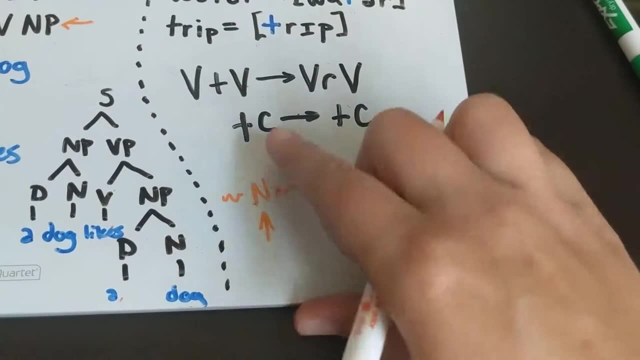 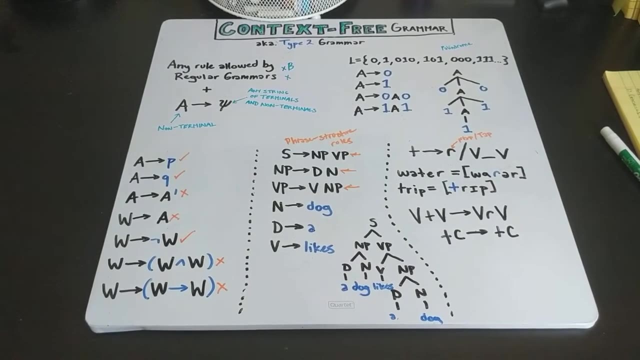 So this is a more going to be a more complicated set of rules, because you're allowed to have anything you want as long as you've got a non-terminal, All right. so this is going to be the next video. This is a. this is the type of thing we can't- cannot do with a context-free grammar, and so we'll need to build a context-sensitive grammar.